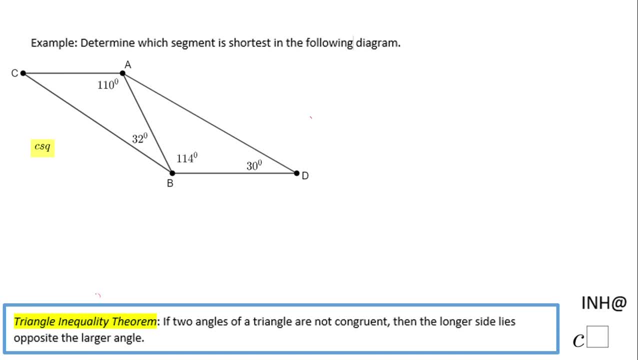 Welcome or come back any help. at C square in this example, we need to determine which segment is shortest in the following diagram. so which of these segments- AC, AB, BC, AD or PD- is shortest? and for that reason we're gonna use this triangle inequality theorem and we're gonna look. we use 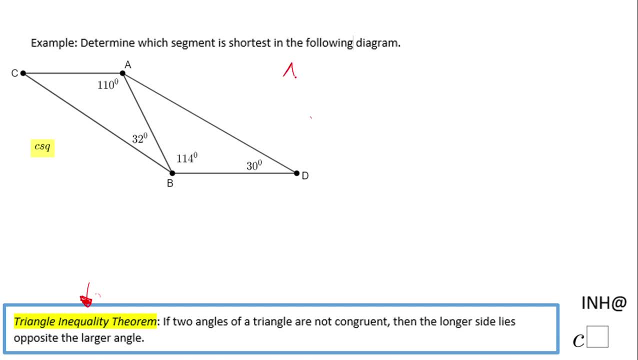 that theorem in two triangles, in the triangle ABC first and then in the triangle ABD. so in order to use this theorem we need to find all the angles. so first of all I'm going to look to how much this angle C is. and if you remember, the sum of the interior angle of a triangle is 180. 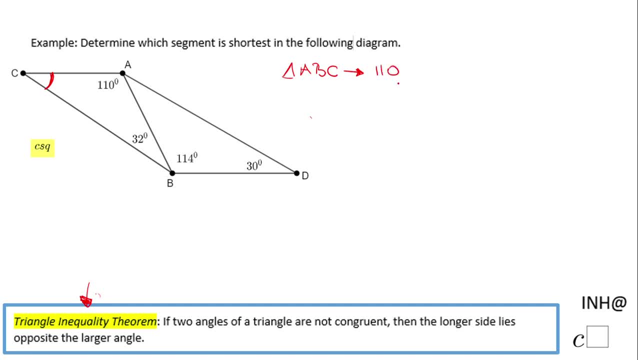 so I'm gonna write here: 110, which is the measure of angle C, AB plus the 32, which is the measure of angle ABC, plus the measure of angle C is 180. I can combine 110 and 32, that is 142 plus the measure of angle C equals 180 subtract 142. 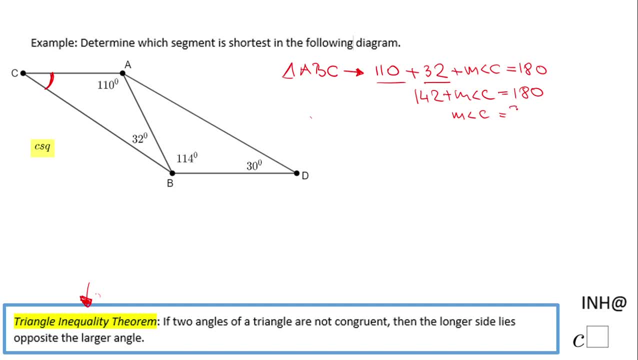 and I have 38 degrees, so this angle here is 38 degree, and now I can look through this triangle and see which side is the shortest. and how can I do that? I'm looking to angles. so this angle is 32 each, which which is the smallest in this triangle. that means 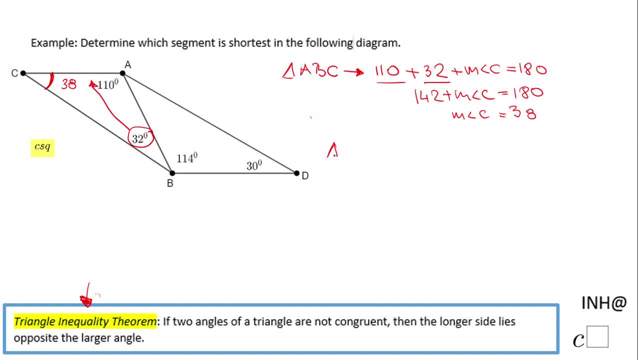 AC, the opposite side, is the shortest, then the next one, the nextığını 38, and means an exciting. this inequality will be AB and the longest. the longest is 27 and this angle of wisht, which is showing us that one inch is always the smallest in this triangle, that means AC is the shortest in every triangle, so that this triangle will look my googunder, which is the. 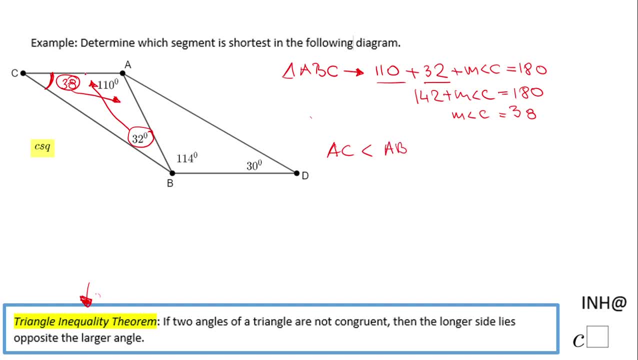 shortest tragic triangle because those angles look Devon, withoutoo. and the longest side in this triangle will be the one that goes to 110, which is BC. We finish with triangle ABC. we're going to move to the next triangle, triangle ABD. 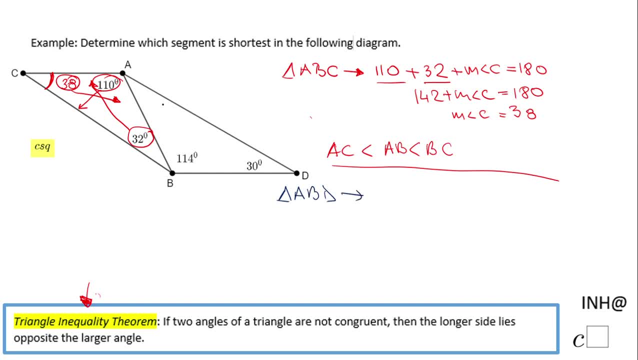 ABD. and the first thing I'm going to do, I'm going to have to find this angle angle BAD. And how am I going to do The same? like here, the sum of the interior angle of an angle of a triangle is 180.. 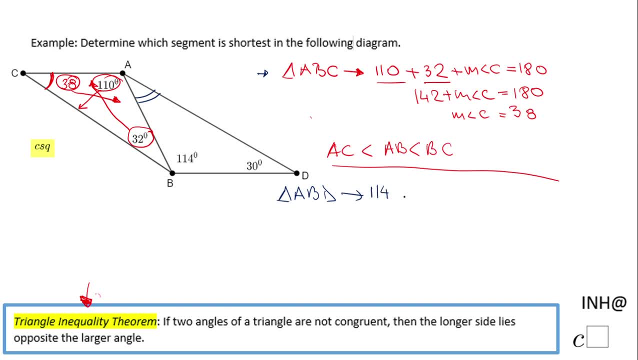 So I'm going to have 114,, which is the measure of angle ABD, plus 30 degree, which is the measure of angle D, plus the measure of angles BAD, equals 180.. We can combine 114 and 30, that will be 144. 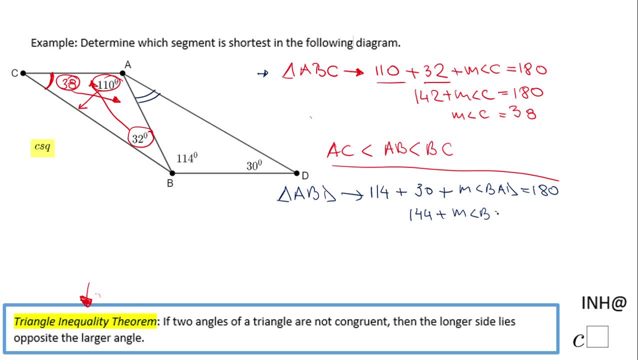 Plus the measure of angle BAD equals 180, and now we can find the measure of angle BAD by subtracting 144, so that will be 36 degree. This angle here is 36 degrees. so now we can use this triangle inequality theorem for this triangle. 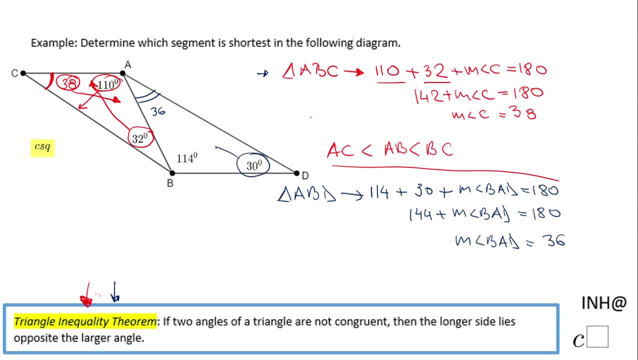 And we notice this is the smallest angle, so the shortest side of BAD And we can see that it's going to be the one that goes of 143.. Then the next side will be the one that goes of 36, right, And that is BD, and the largest side is going to be the one that goes of 114, which is AD. 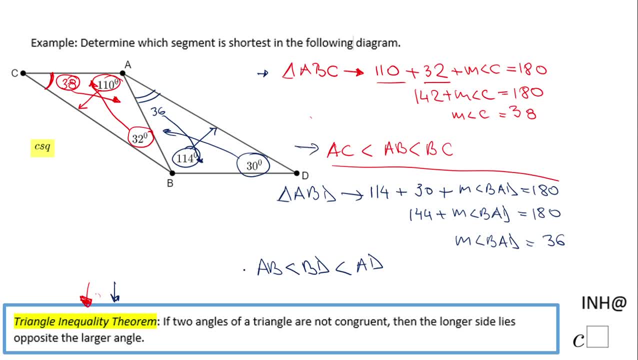 And now the only thing we have to do is to combine these two inequalities. Take a look at which one is the shortest by comparing these two inequalities And, in fact, if you take a look here, we can connect these two inequalities using this first part. 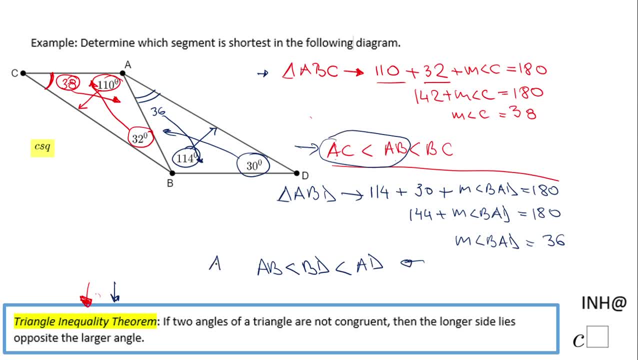 AC is less than AB, AC is less than AB. So now we look in here, we know that the shortest side is AC. AC is the shortest, And that's it. If you enjoyed this video, don't forget to click the like button. And come back on C-squared for more help. Thank you.